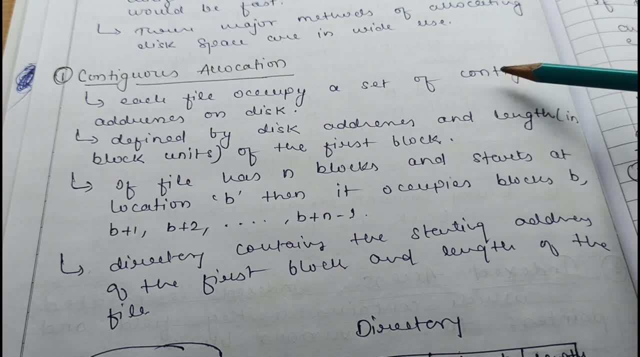 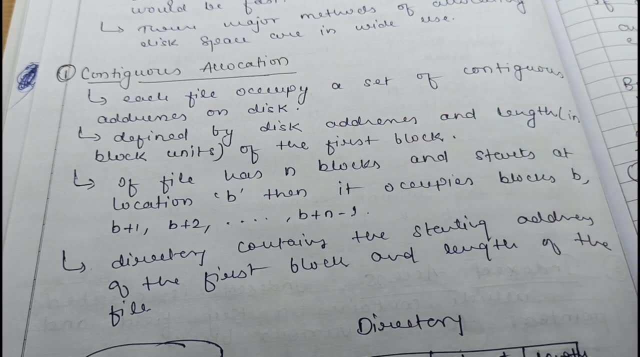 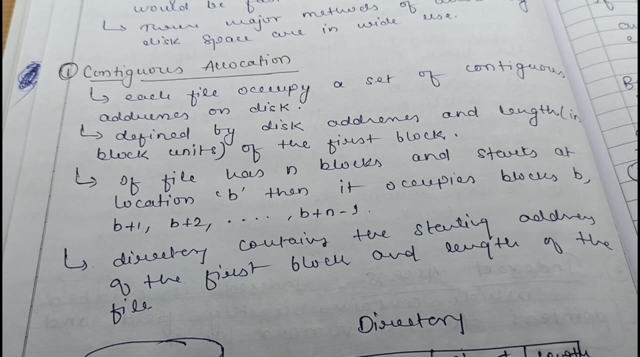 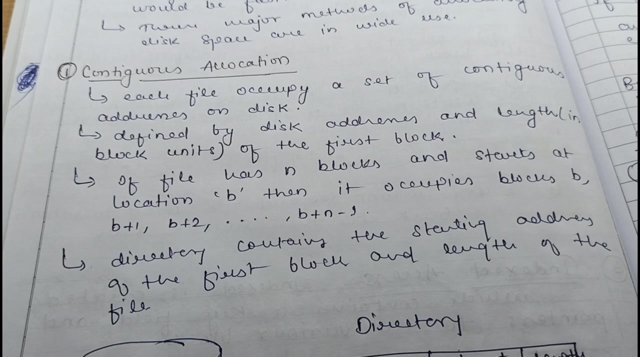 That means a set of contiguous blocks will be given to a single file- Okay, Defined by disk addresses and length in block units of the first block, The disk addresses define a linear ordering on the disk, Like if you are providing contiguous blocks to any file and one file has n blocks. 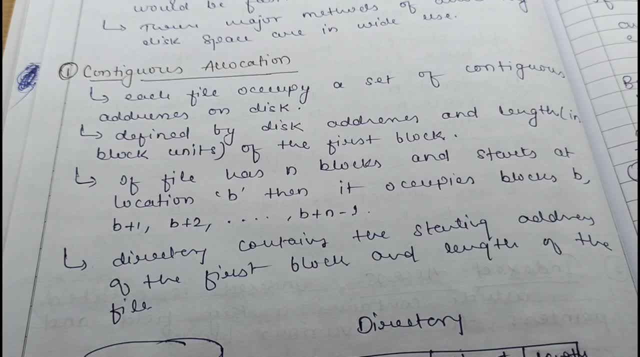 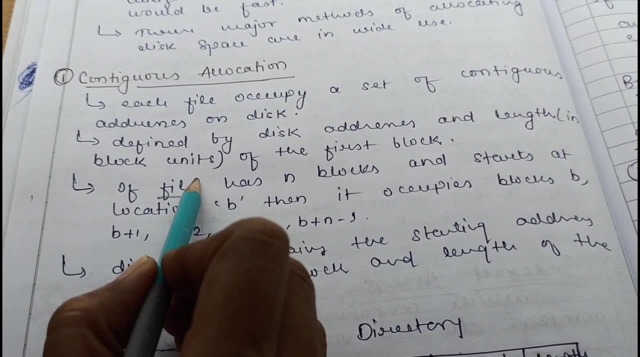 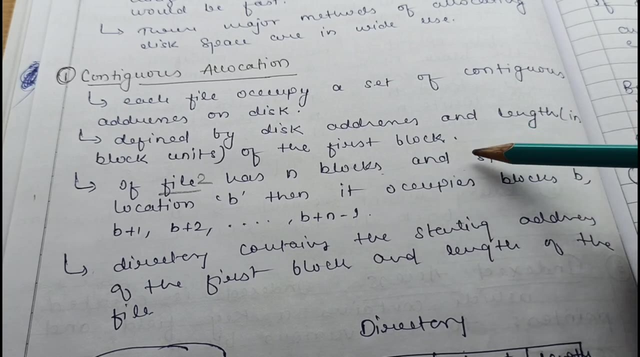 Okay, It is not necessary that it gets only the 0th block at the starting. Okay, Before that it may be possible that there are many more files. So the file, like a file 2, has come and it gets n blocks and it is the first block. starts at location B. 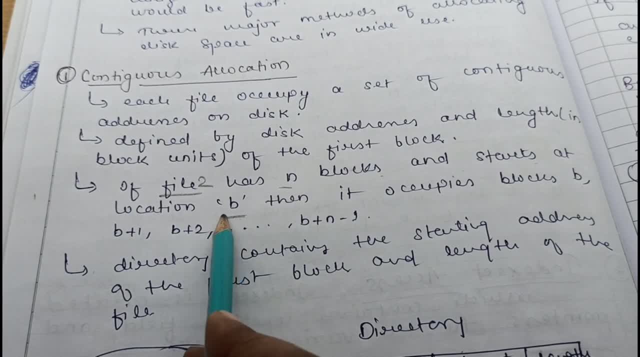 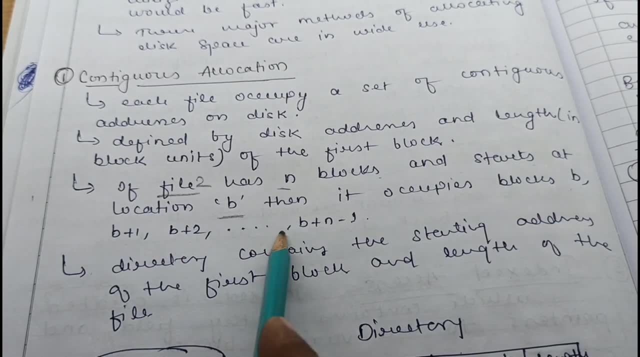 So, and you have given it n blocks and it is starting from B. So what will happen? How many set of contiguous blocks will there be? B, the first one, B plus 1. B plus 2. So on. 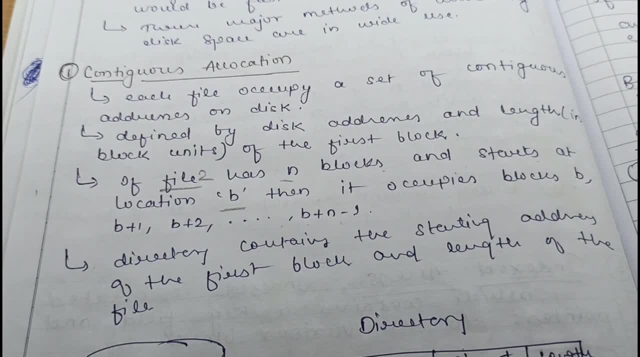 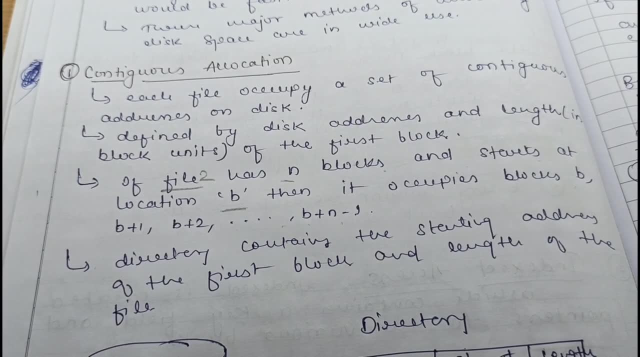 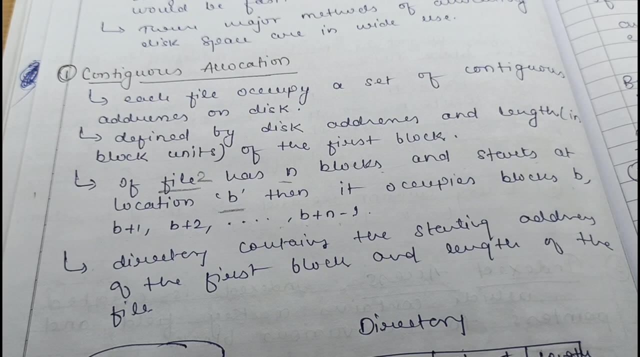 B plus n minus 1.. So these are the different addresses. disk addresses for a block will be given to the file number 2.. So when you will keep a directory structure about this file, the directory contains the starting address of the first block and the length of the file. 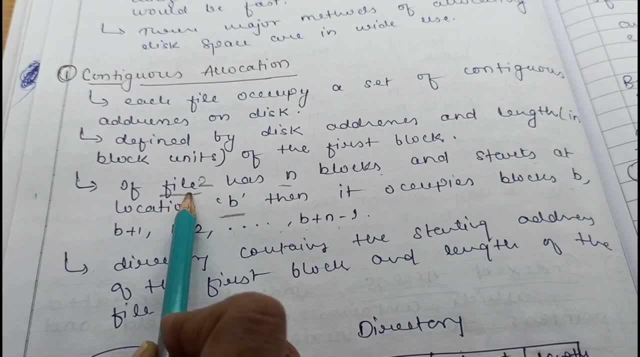 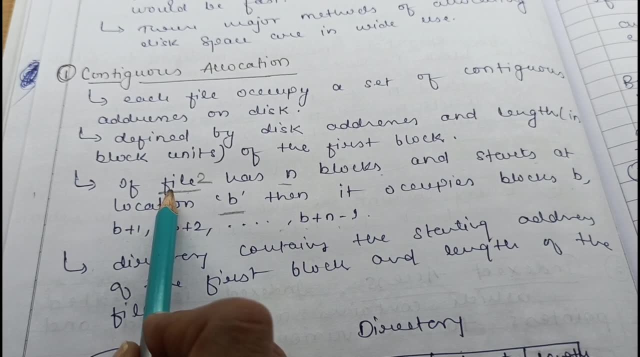 Okay, So file. we have read this first File. In system we maintain an entry of every file. we keep a directory entry That maintains the directory structure. So when you are making the directory entry for this file, it will contain the starting. 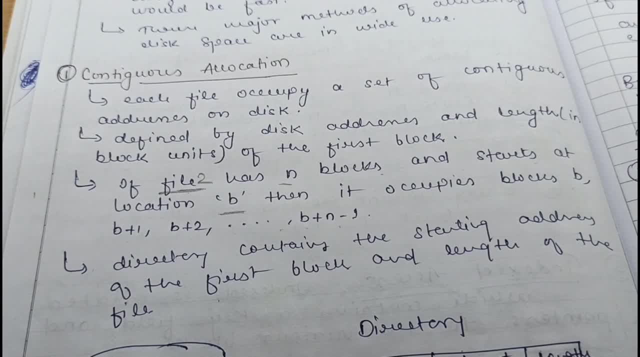 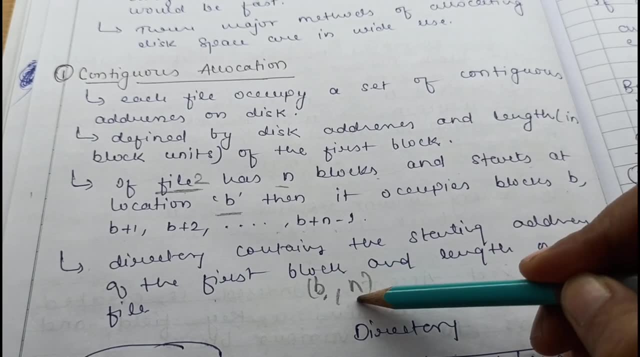 address of the first block, That is B, And the length of the block, that is n, So B n. The directory entry will be like this: It has started from B block and the length is n. Okay, So in this way. 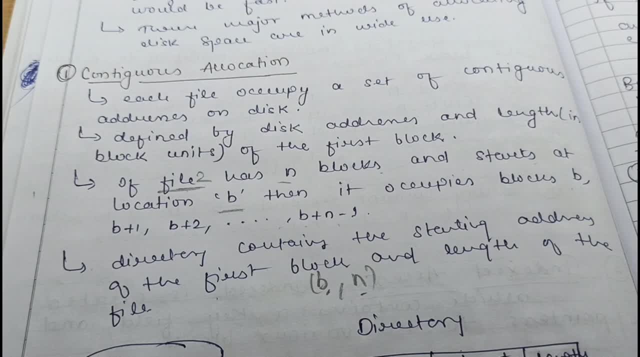 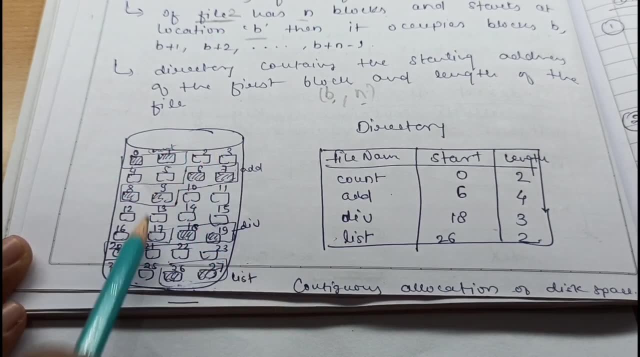 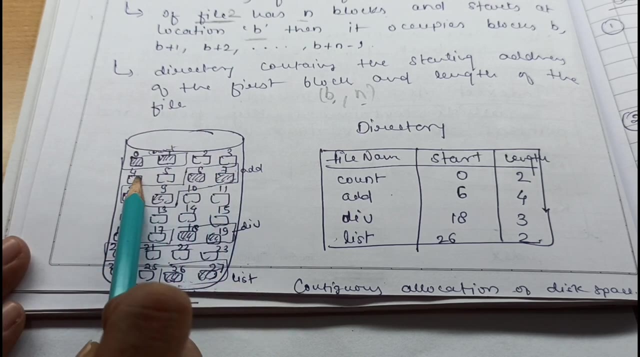 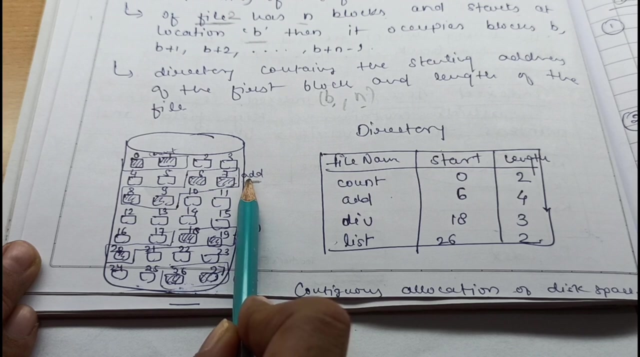 In contiguous allocation we assign blocks to files like this. you can see, just assume this is a disk. it has several blocks and some blocks are free and some are allocated. the shaded one are allocated, so the one like there is a function, add function, we have to give, we have to store this function. 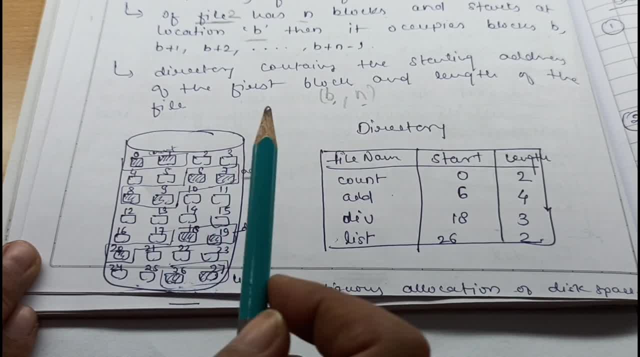 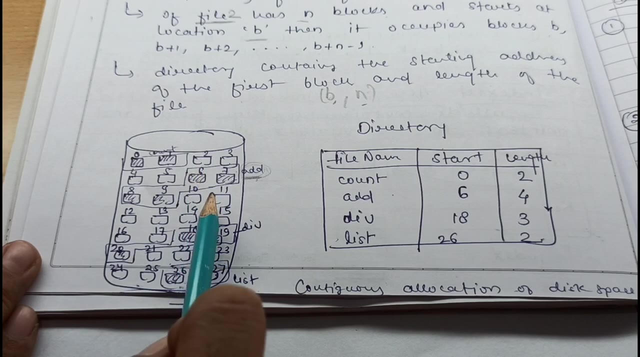 or this file: add file where the function source file ho sakta hai, this function ko store karna hai. toh ye file jo hai. hamne usko four blocks diya hai, aur because it is contiguous allocation, you have given six, seven, eight, nine direct blocks of contiguous allocation. toh dekho. 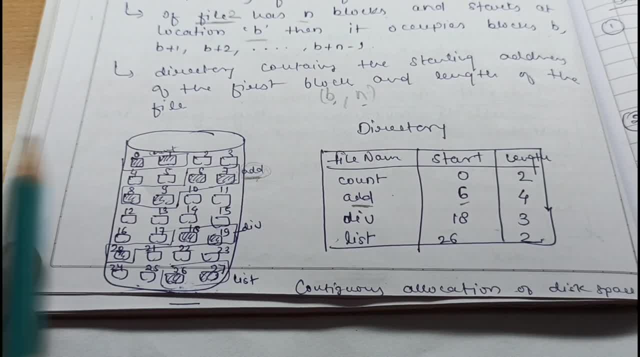 add ke liye, We have kept the starting address as 6 because it has started from the 6th block. and how many blocks have been given to them? 7,, 8,, 9, total 4 blocks, So length is 4 blocks. 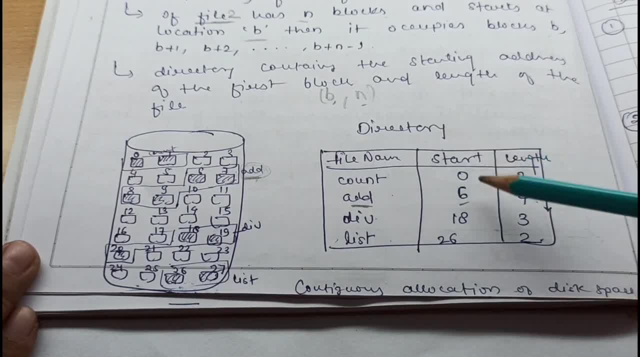 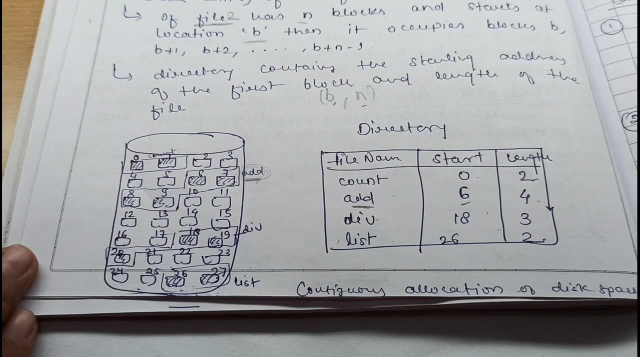 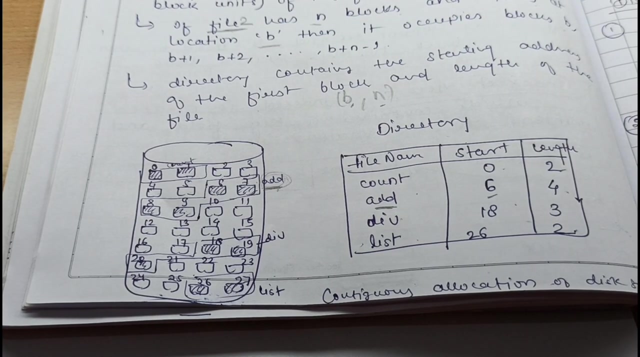 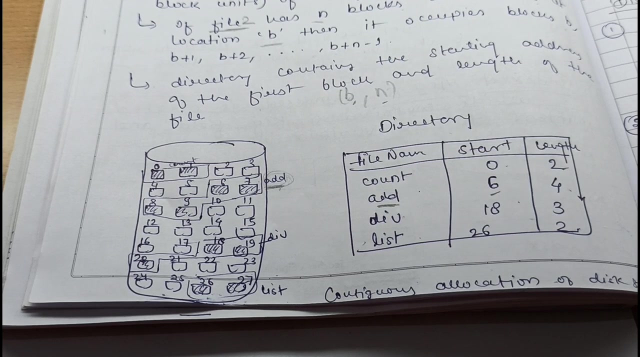 So, likewise, how will the directory entry of all the files be maintained, The starting block address and the length of the file? Okay, So in this way contiguous allocation is maintained in our file allocation method. So tell me one thing: if we have stored the file in disk with contiguous allocation, now if we have to access the file, then we have read 3 access methods. 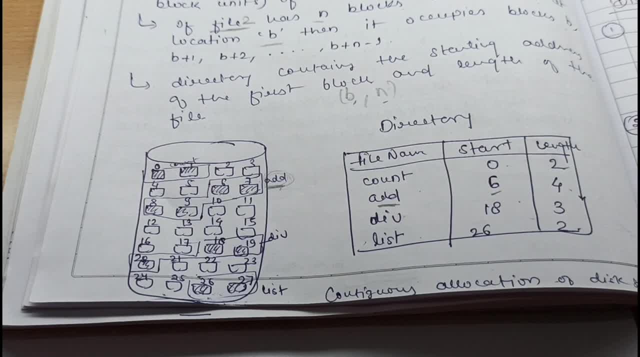 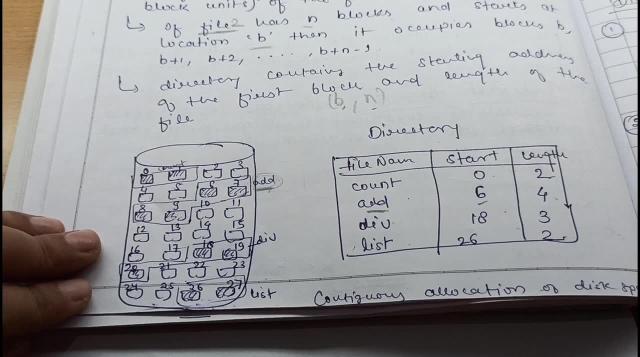 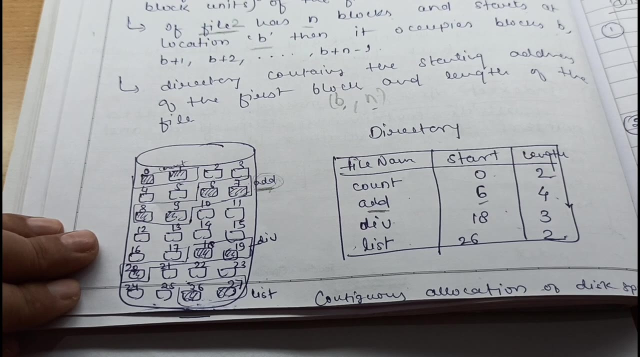 So first is sequential access. Is it possible to access this file sequentially Which is storing contiguous? So you just need to know the starting address and the length so that protection is also done. then you can easily access the file sequentially. Okay. 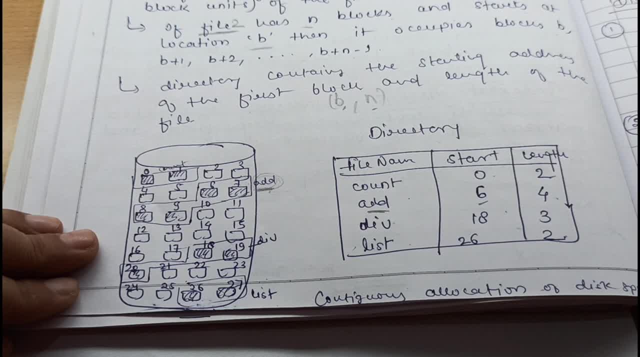 So file system remembers the disk address of the last block as far as it has read and as soon as it has to read next, it has to do it sequentially, as and when required. reads the next block, And if you want to access directly, then. 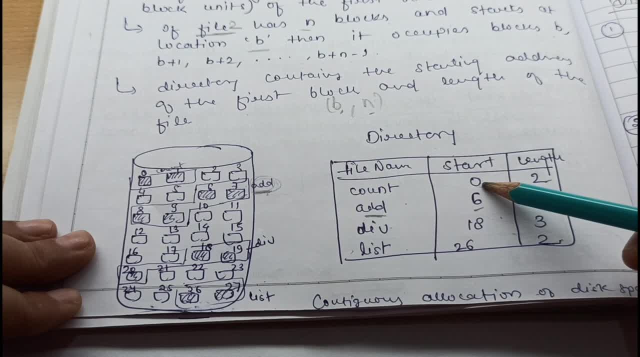 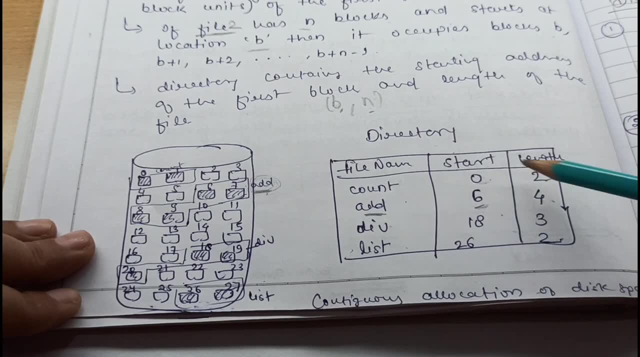 So we have to do this. We know the start block and we have to go to the third block. the user has told us that we know the third six starting. we want the third block. we want the third block. that means, which block will you go to next? 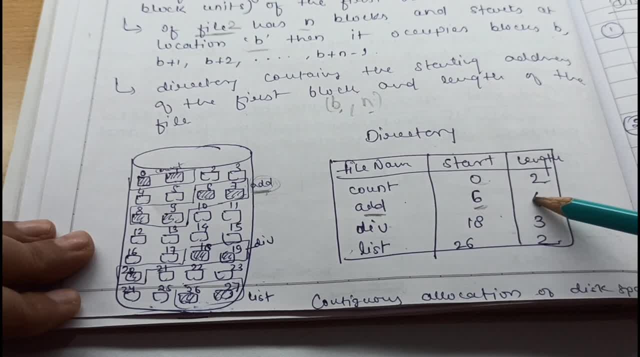 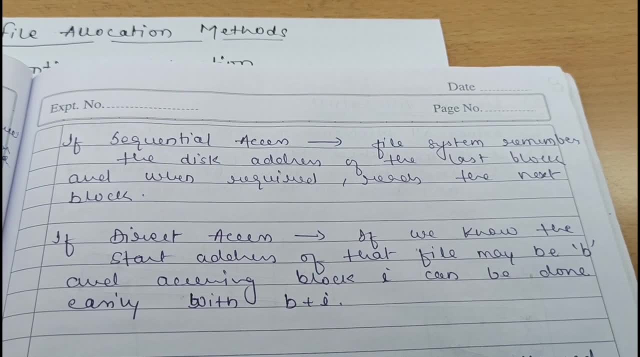 So you will go to the block of the disk from the absolute address where the actual data is present. so in contiguous allocation both the sequential access and direct access method is possible. So in contiguous allocation both the sequential access and direct access method is possible. 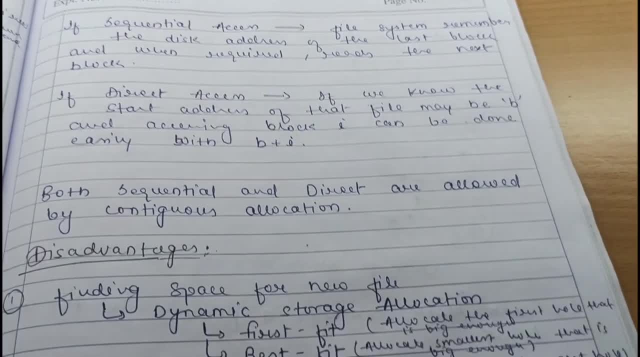 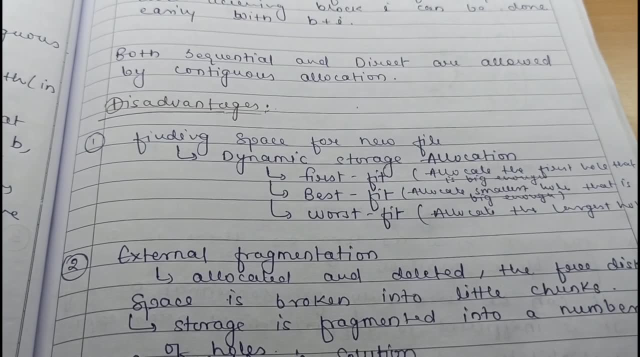 So in contiguous allocation both the sequential access and direct access method is possible. Okay, So both sequential and direct access methods are allowed by contiguous allocation. So what are the- what can be- the disadvantages of it? I wrote some of them. 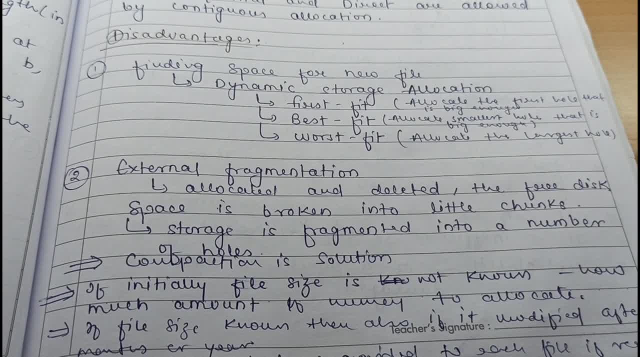 First one. Now, if you are talking about contiguous memory allocation, then we had read: memory management First fit, best fit, worst fit. that is the same thing. So, finding a space for the new file, you can use dynamic storage. 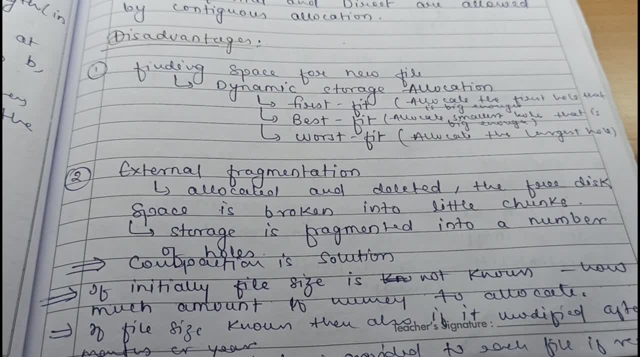 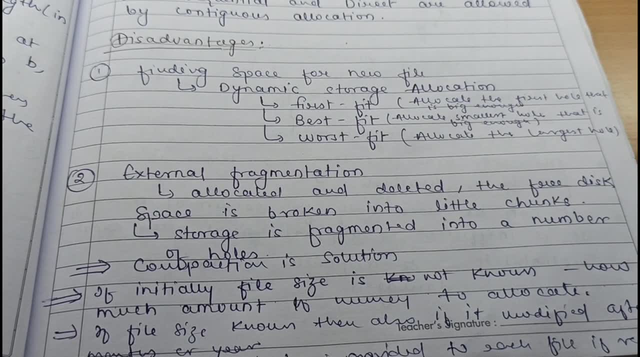 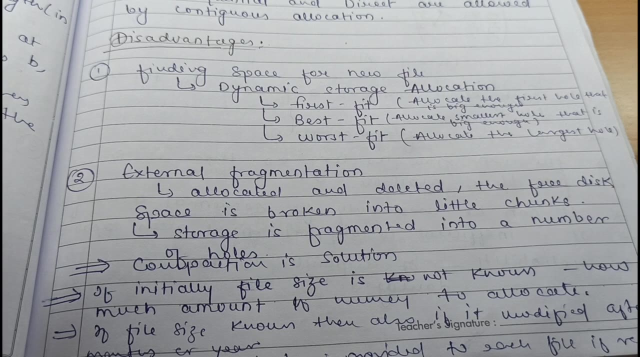 As I said, you can use dynamic storage allocation. Any of these can be used. But what was happening in all of these? External fragmentation was happening, And in some it is internal also. How external fragmentation is done: Contiguous allocation is done. A file is deleted from B Its space is left empty. That file becomes chunks of such small free space When you compact. the compaction happens. So if you put that set of blocks in free space blocks, then it is fine. If it is not done, then these small chunks, memory chunks, free memory chunks that cannot fulfill the demand. 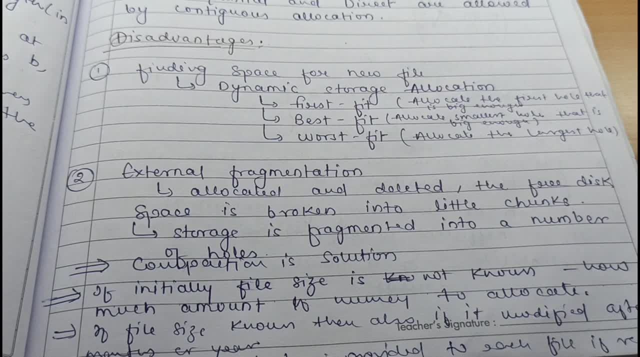 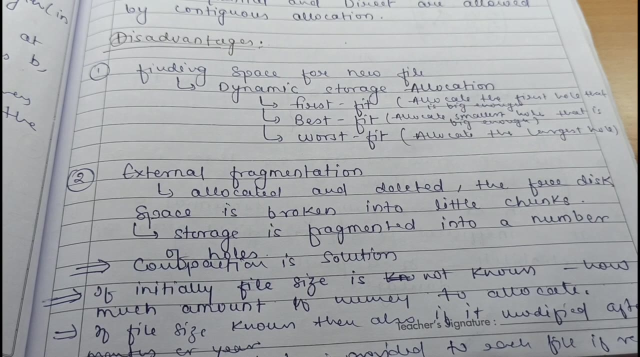 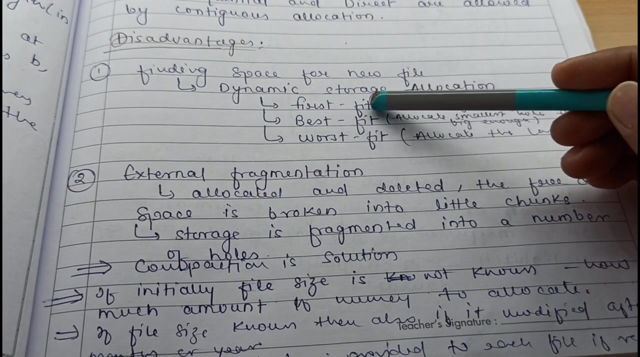 of new file which is larger in size than the smaller chunks. So because of this, external fragmentation can happen here too, Because we are talking about contiguous allocation. So compaction is a solution that I wrote here. There will be one more problem here. If we choose worst fit, best fit, first fit, Let's. 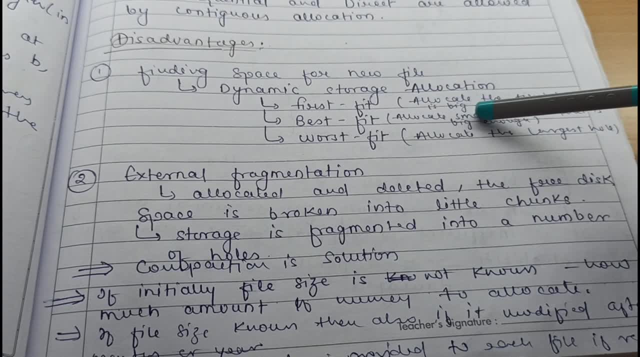 choose best fit. So what happens in best fit? It allocates smallest hole. that is big enough. So this means that we know the size of the file initially. If initially file size is not known, then you don't know how much amount to allocate or how much amount of blocks or 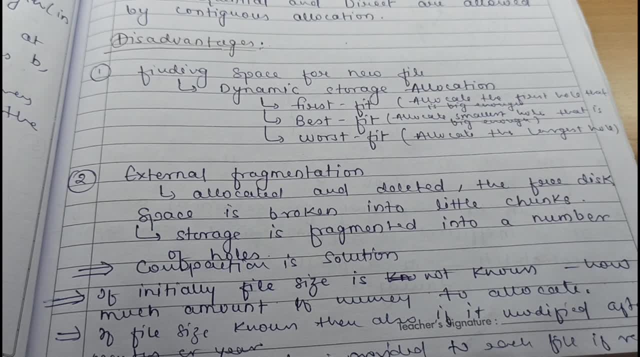 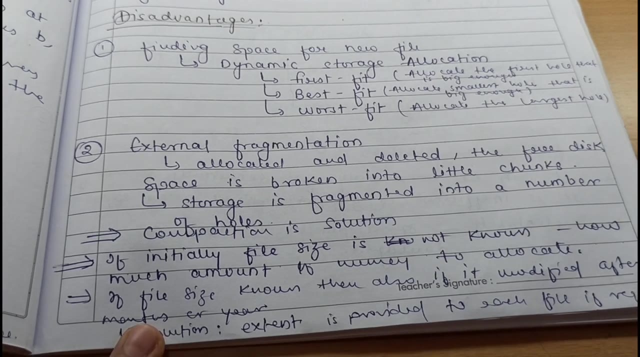 how much amount of memory. If it is not known, then you cannot allocate the exact amount of memory to that file And in future, if its size increases, then you cannot give it because you have set of contiguous allocation, allocated blocks. It is actually not possible now. 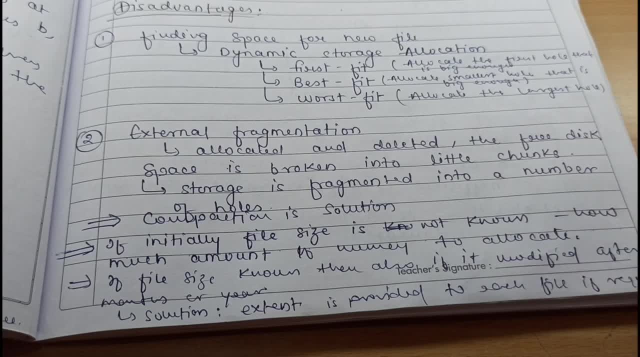 And what would happen in worst fit? If you have given worst fit, then our internal fragmentation can happen too. Okay, so you have given more than what is required. You can make file size bigger. yes, that's what it is. So what about final fragmentation? 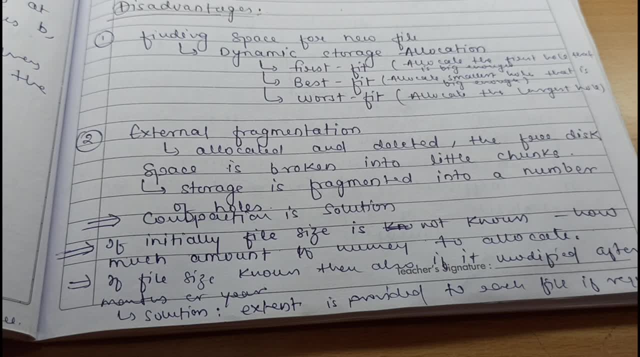 the size of the file has never increased. the size of any file will increase. the size of any file will not increase, so you can't put all of them in the worst fit. otherwise it will be a problem with external fragmentation. internal fragmentation will also happen, right?